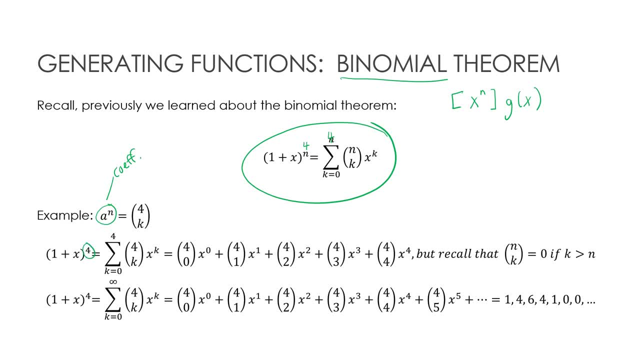 And again, 4 came from the fact that n is 4.. So 4 choose 0,, 4 choose 1,, 4 choose 2,, 4 choose 3,, 4 choose 4.. But let's say I want to keep going because let's say I have 4 choose 5,, 4 choose 6,, etc. 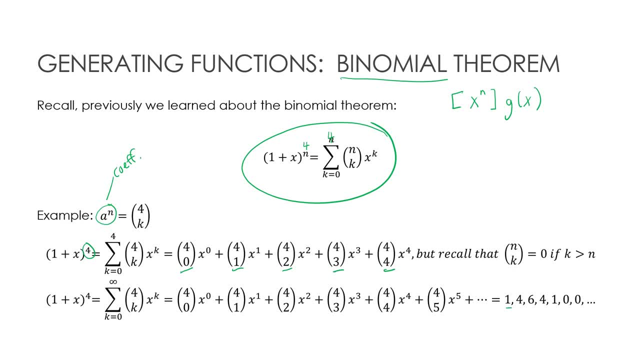 Well, what's going to happen? I'm going to get my 1. Which is 4- choose 0,. 4- choose 1 is 4, 4- choose 2 is 6,. 4- choose 3 is 4, 4 choose 4 is 1.. 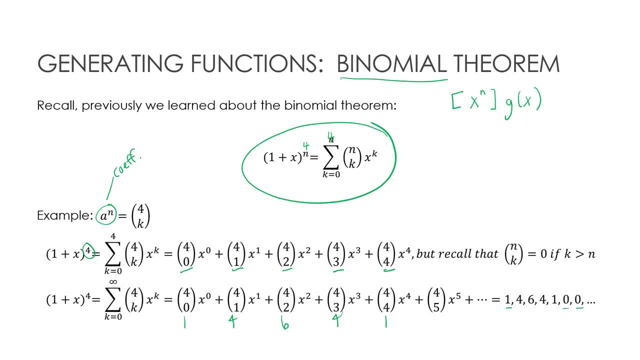 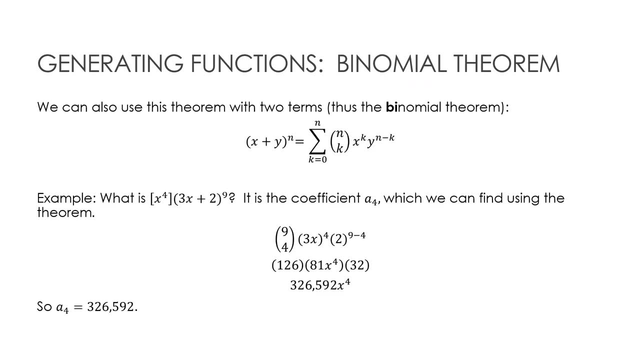 Anything where k is greater than n is going to result in a 0.. So this would be the series that I would come up with using the binomial theorem, And because this is, of course, the binomial theorem, that of course means that I don't have to have one of my terms be 1.. 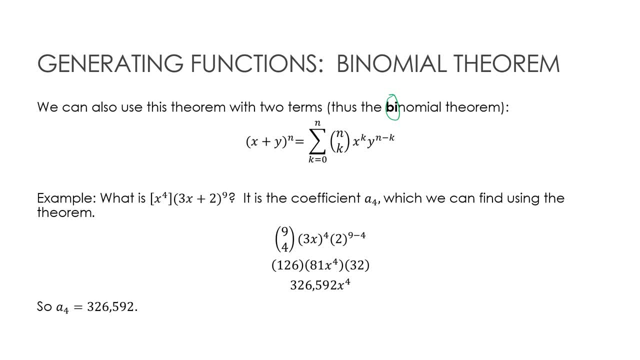 I could have two variables, Or I could I could have the 1 be some other number. So essentially I'm looking at two terms instead of just one, And essentially that means that whatever the first value is is going to be to the kth power. 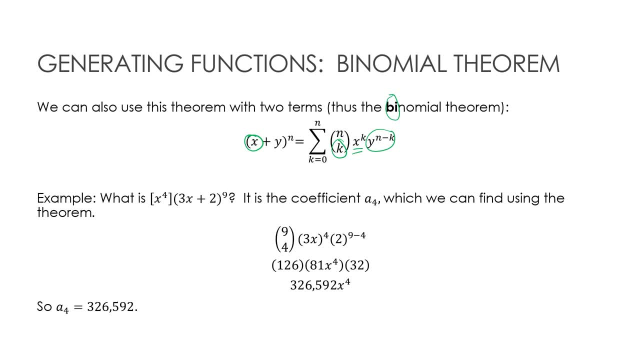 And whatever the second value is is going to be to the n minus kth power. So, for instance, using the binomial theorem, let's say I wanted to solve this. I want to know, And again, what? What does this mean? 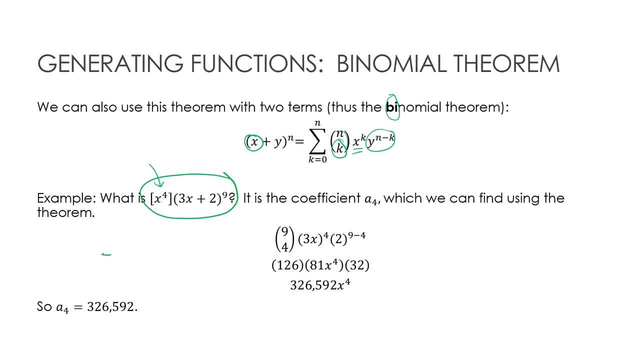 That means what is the coefficient in front of x to the 4th? if I were to multiply this out, 3x plus 2 times, 3x plus 2,, 9 times Now this would be a pain in the butt if I did this 9 times. 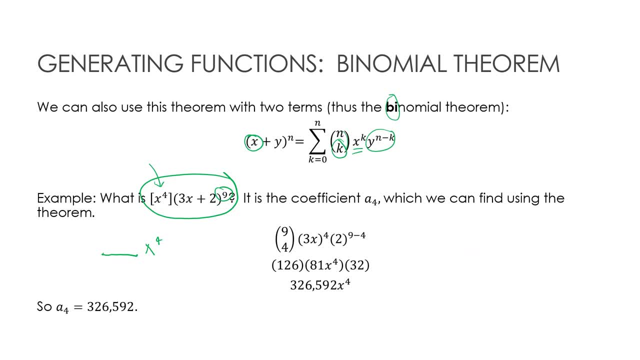 So instead let's use the binomial theorem that says: hey, do this, This is 9, choose 4.. So that's 9 factorial over 5 factorial, 4 factorial, which turns into 126.. And then x to the k. 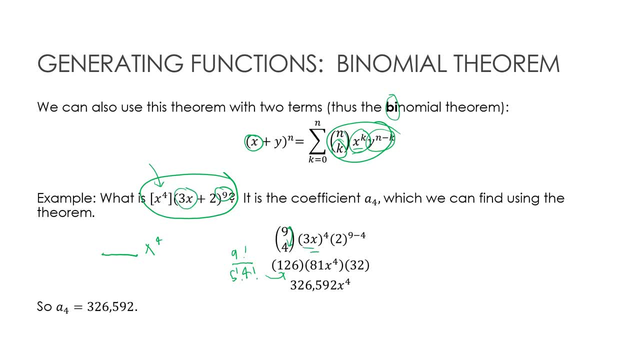 So that's 3x to the 4th power, And so really I'm saying 3 to the 4th, which is 81.. And then y to the n minus k, So 9 minus 4 is 5.. 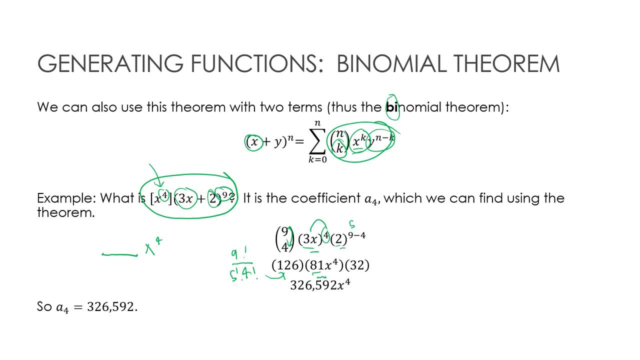 So really I'm saying: take 2 to the 5th power, And 2 to the 5th power is 32.. If I multiply 126 and 81 and 32, I get 326,592 and x to the 4th. 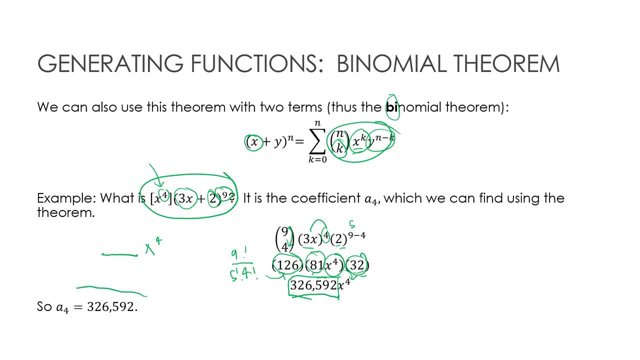 So what am I interested in The coefficient? That's the answer that I'm looking for. Again, instead of multiplying it out, I just use the binomial theorem. What I want to do now is take a look at the same binomial theorem. 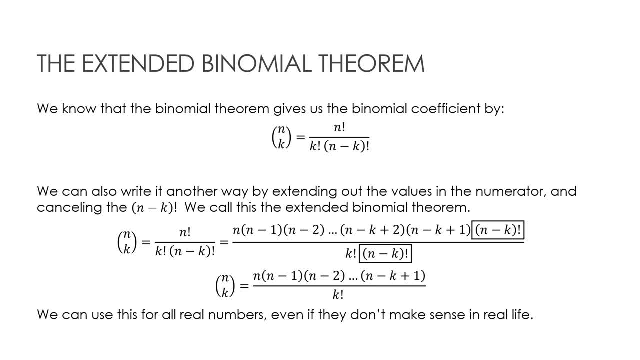 We're not changing anything, but we are going to write it a little bit differently. It's still the same theorem And I want to use it for things that maybe don't make sense in real life. So, for instance, if I wanted to choose negative 3, choose 2, or 1 third, choose 4.. 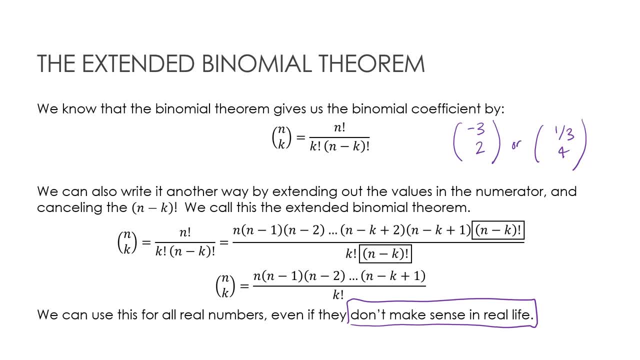 Those things don't make sense in real life. But you'll see once we get to where we're putting this all together, Why we need this extended binomial theorem so that we can calculate ideas like this. So here's our normal binomial coefficient. 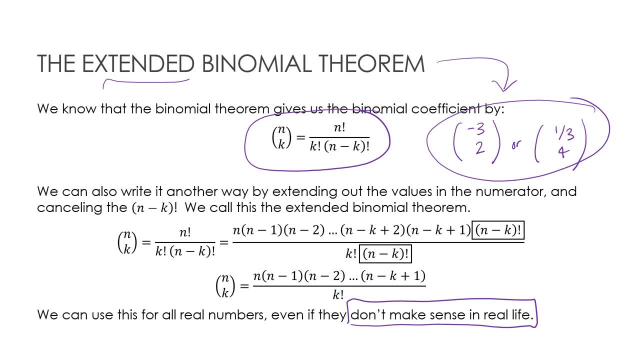 And choose k is n factorial over k factorial, n minus k factorial. Now, as you can see, if I take the numerator and I just start expanding it, n factorial means n times n minus 1, etc. And I keep expanding that all the way to n minus k factorial. 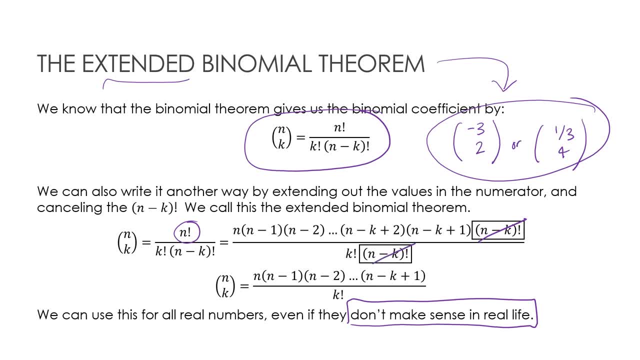 Then at some point I'm able to cancel that n minus k factorial on the top and the bottom, which leaves me with this, And so essentially what I'm saying is n times n minus 1, etc. all the way down to n minus k plus 1 over k. factorial is another way to write this. 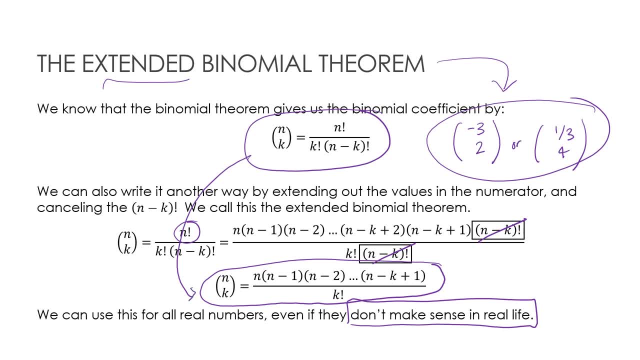 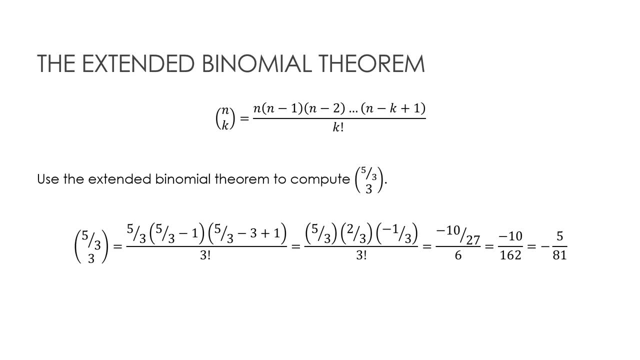 Now, when would I do it? that way? I'll show you. Say: I want to find 5 thirds, choose 3.. So what I'm saying is: start at 5 thirds, then take 5 thirds minus 1, then take 5 thirds minus 2, etc. 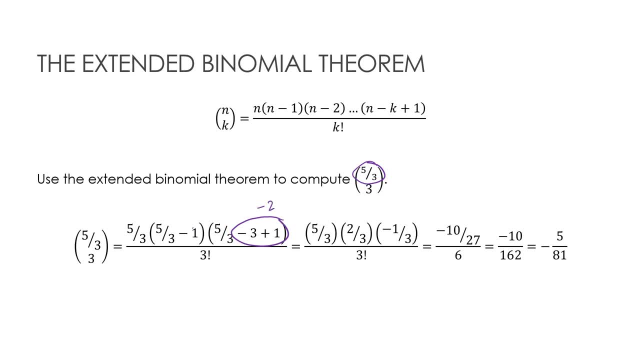 Now, obviously this is the same as minus 2.. And if you're confused about how many places to go to remember, we're choosing 3.. So I'm going to have 3 terms on the top here. So it's 5 thirds times 2 thirds times negative 1 third. 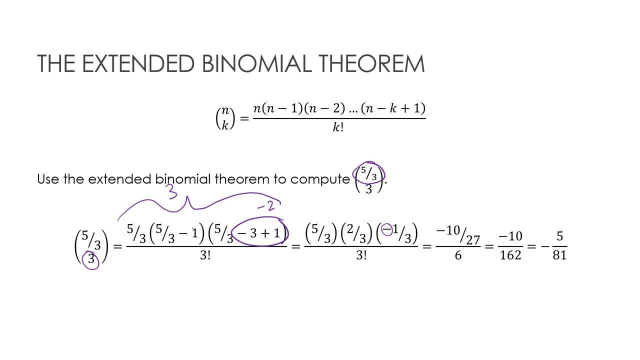 And don't get freaked out by the negative That's going to happen. The denominator is still k factorial now, So 3 factorial. So if I multiply all of that out, I have negative 10, twenty-sevenths over 6,. 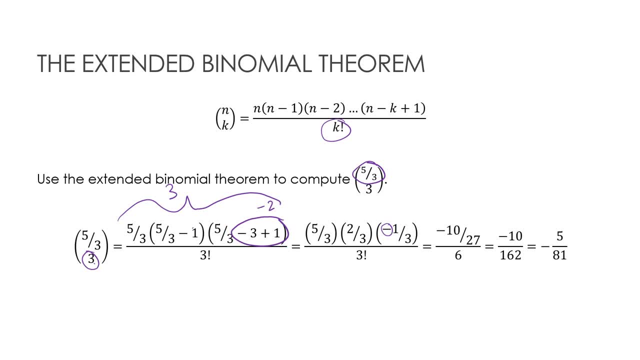 which is negative 10 over 162, or negative 5 over 81. Now again you might be thinking she's lost her mind. Now I've got a negative value. but again, I promise you this will make sense. 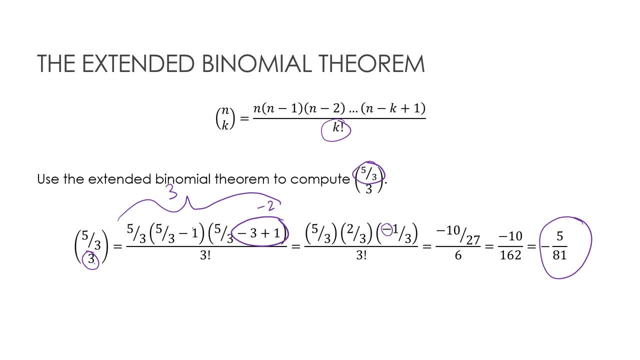 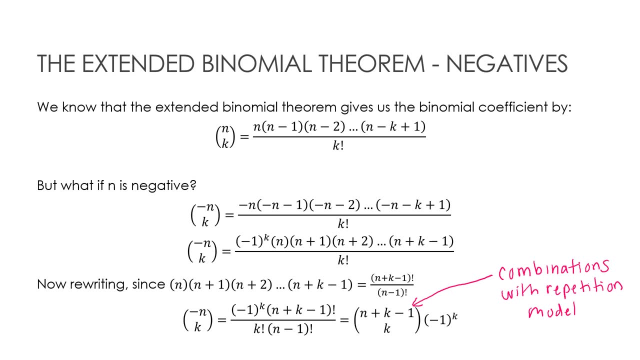 once we get to the point where we're actually using this in a question. Let's take a look at another example. I've rewritten the extended binomial theorem for you at the top, But the question now is: what if n is negative? 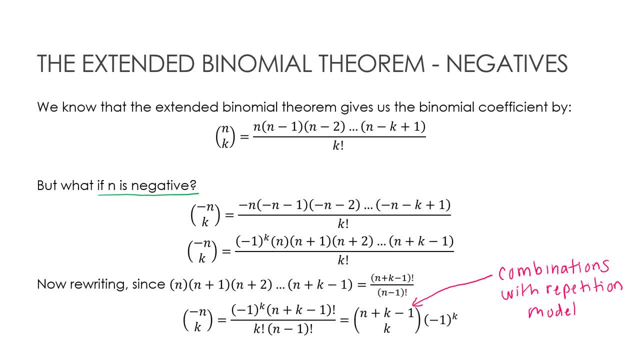 Negative n, choose k Again. does that make sense in real life? No, I can't have negative 7 of something. choose 2,. but in mathematics it can make sense If we're just applying a formula. So think about if I had a negative n. 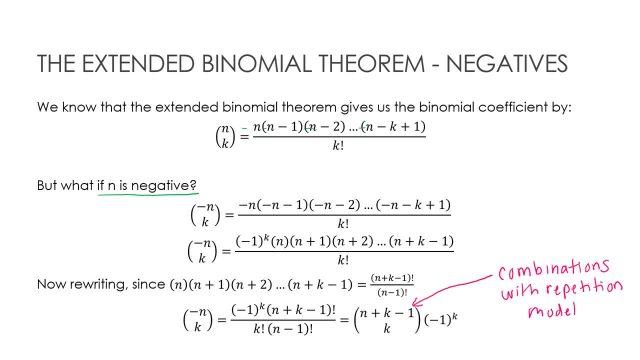 Really, I just have a negative n on all of these values, which I can then factor out the negative. So essentially, I'm factoring out the negative How many times k times, because that's how many values I have in my numerator is k values. 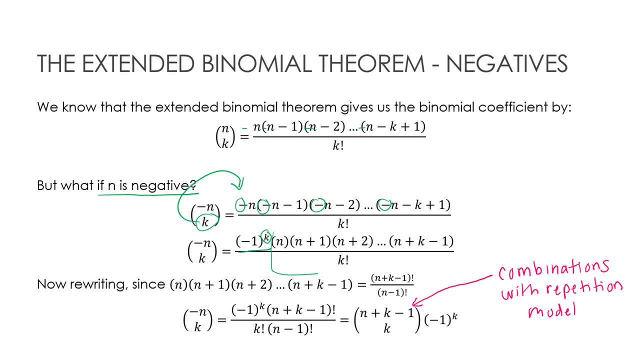 So negative 1 to the k and then all of this Which looks like this- And if you'll notice, this part is just my combinations with repetitions: model n plus k minus 1, choose k, Which is super interesting. 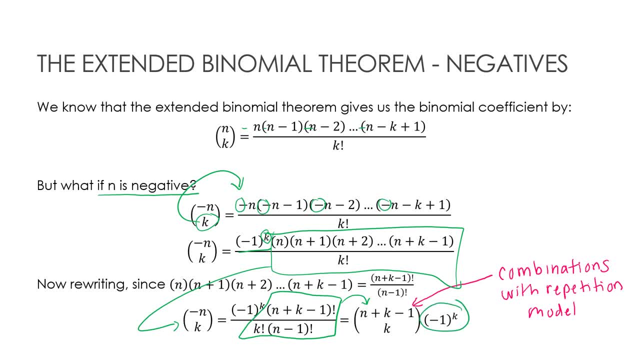 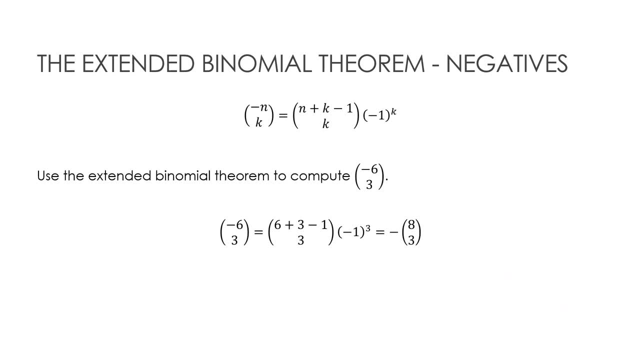 And then, of course, we just have to take it times negative 1 to the k, because that was not part of our original function. Let's take a look at how we might use this. Let's say I wanted to expand negative 6, choose 3.. 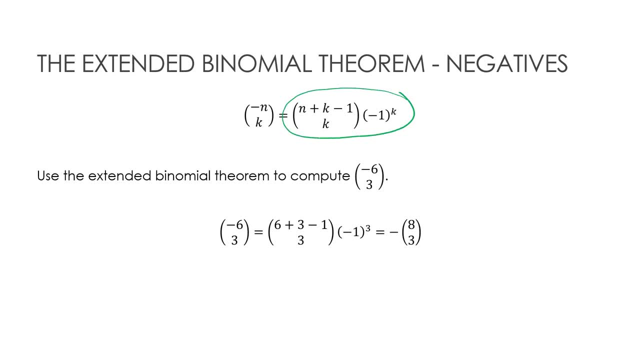 So negative 6, choose 3.. Again, using this extended binomial theorem for negatives, I'm saying: let's take n, positive n, which is 6, plus 3, minus 1, choose 3.. And then, of course, negative 1 to the 3rd. 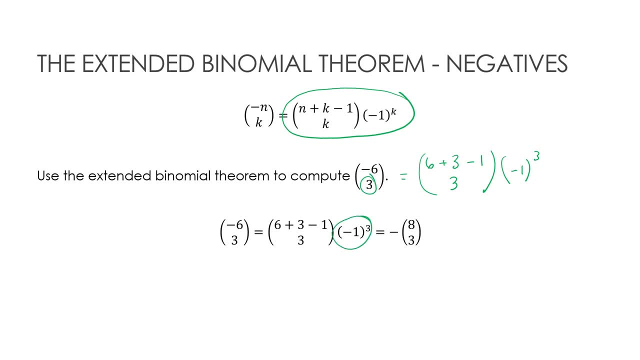 Now we know negative 1 to the 3rd Is really just going to be negative 1 to the 3rd. So negative 1 to the 3rd is going to give us a positive or negative based on if it's an odd or even k value. 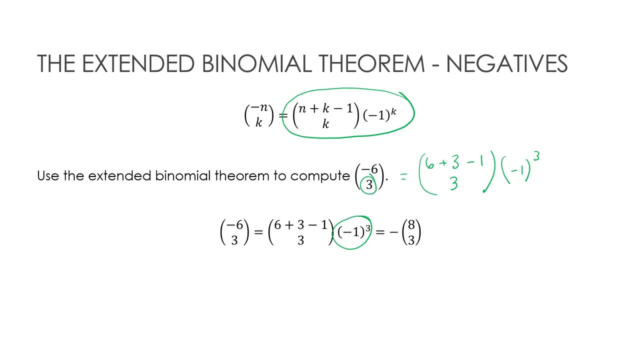 So, obviously, if it's an odd k value, our answer is going to be negative. If it's an even k value, our answer will be positive. So what I have here, then, is 6 plus 3 is 9, minus 1 is 8.. 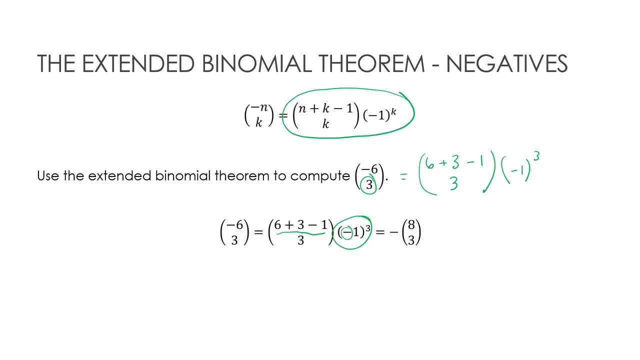 8,, choose 3.. And of course the answer is going to be negative, because negative 1 to the 3rd is a negative 1.. So there's my solution Again. could I go ahead and find that solution? 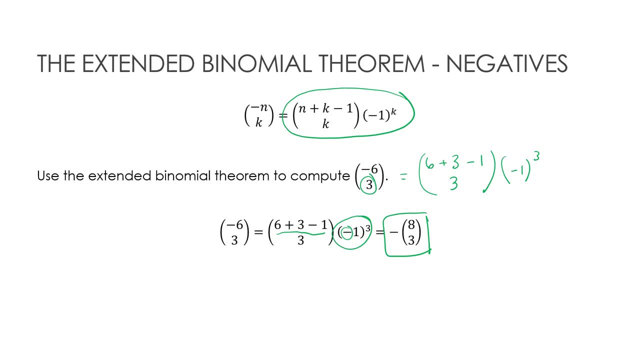 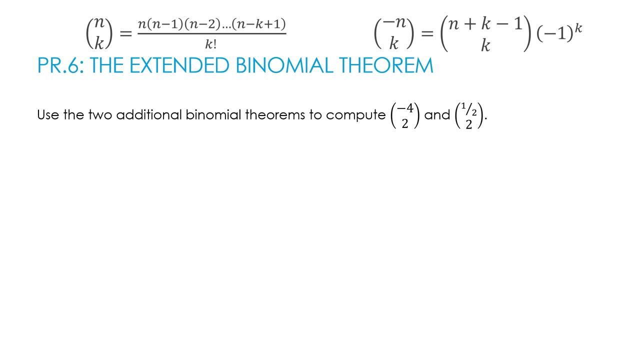 Of course, But we're more interested in computing or showing the correct way to find it, as opposed to actually getting your calculator out to find what 8, choose 3 is Before we start using these theorems in actual questions. that we're going to do, and I promise I'm going to put it all together for you very soon- 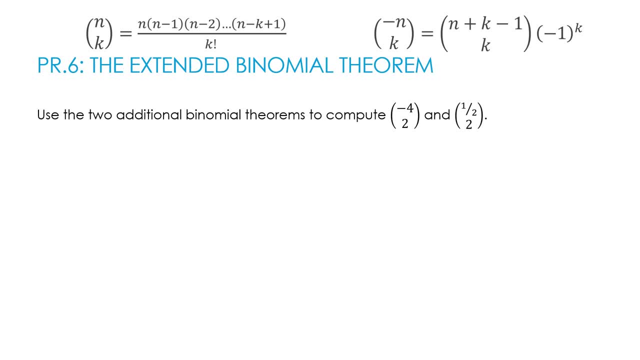 I want you to just practice using them so that that's not a stumbling block When we get to, of course, the hard part, where we actually put everything together For the first one. and again, I encourage you to press pause, try both of these questions and then press play to see how you did. 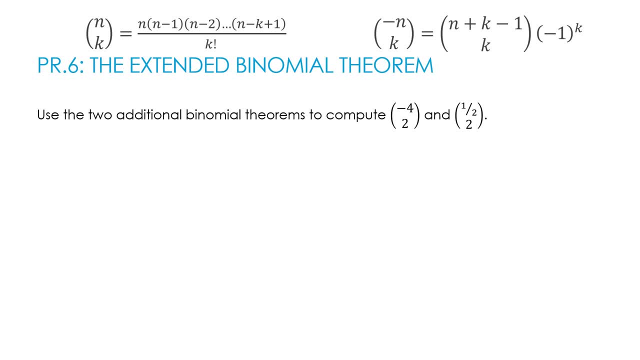 For the first one I'm looking at a negative value, So again I'm focusing on this one, And this one says: take 4 plus 2 minus 1 over 2.. 2, or choose 2, and then negative 1 to the second. 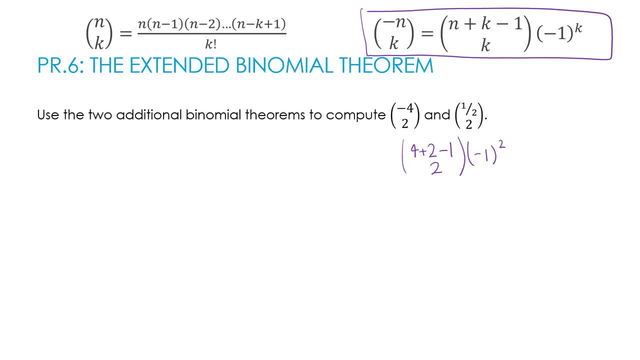 Now do I care about the negative 1 to the second? Negative 1 to the second is going to be positive 1.. So I really don't care. So what I'm ending up with? and you can go ahead and write negative 1 squared. 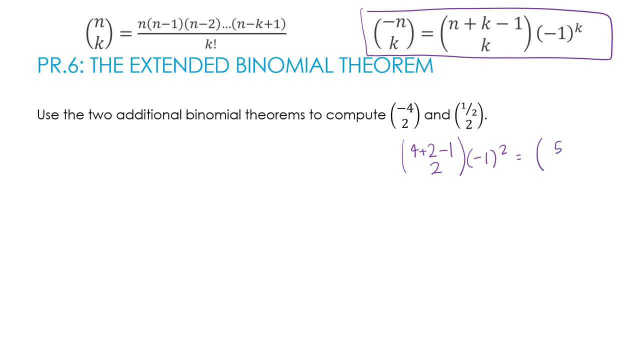 4 plus 2 is 6, minus 1 is 5.. So my answer is really just 5, choose 2.. For the second one- and again I've already uncovered the answer here, Obviously, but I would just look at this: 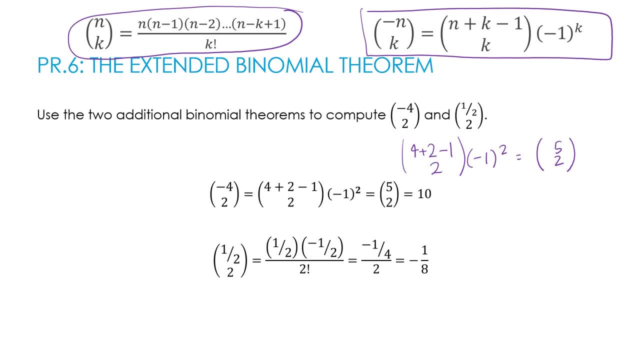 This extended binomial theorem 1 half choose 2 means I start at 1 half. I'm having two values, So 1 half minus 1 is negative. 1 half over 2 factorial, That gives me negative 1 fourth divided by 2, which is negative 1 eighth. 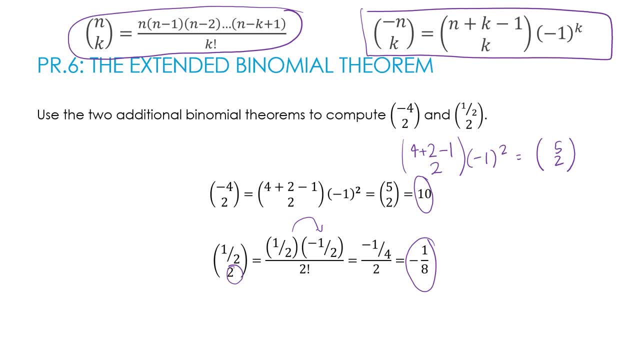 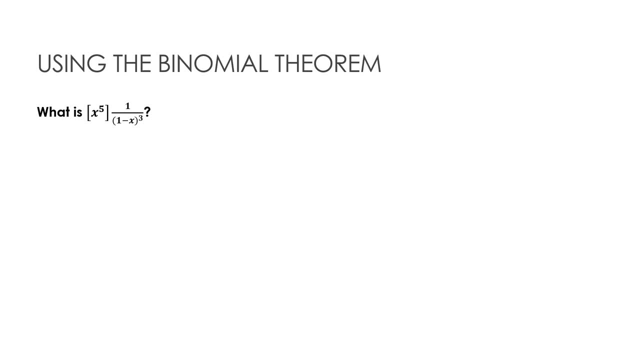 So you can see I have found both of my values. We are almost there. So when we put this all together, I'm actually just going to give you the story problem And then you're going to have to do what we did in section 9-1,. 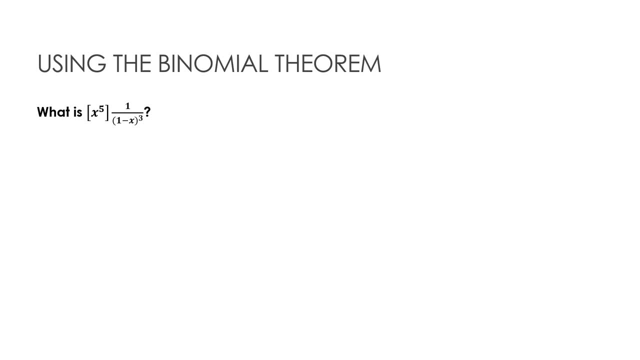 which is come up with a generating function, And then all of the stuff we've learned in 9-2 so far, which is rewrite that series in a more I don't know easy to deal with way like this, And then use that to find the actual coefficient. 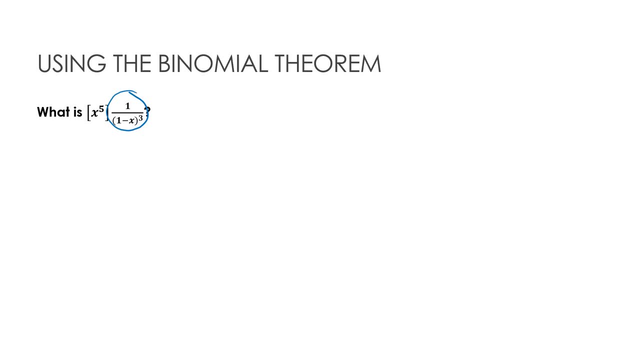 So use all of these strategies that we're talking about. So we are almost there. We're just going to put it all together in a little bit, But here's a really good pre-trial. We're going to do a little bit of a review. 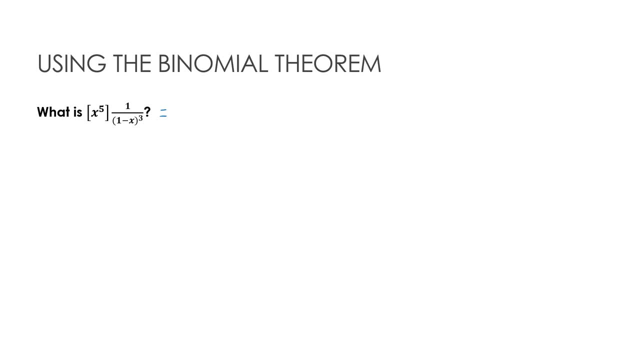 The first thing I would do here is remember. this is telling me I'm looking for the coefficient of x to the 5th. I'm going to rewrite 1 minus x, 1 over 1 minus x to the 3rd as 1 minus x to the negative 3rd. 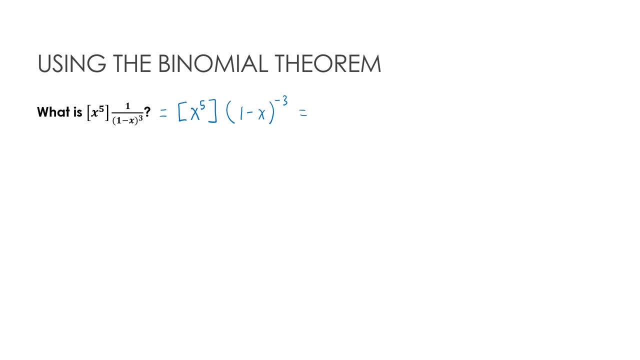 Now, what I just learned about dealing with negatives tells me that this is going to be negative 3. Choose 5.. And then I'm going to have negative x to the 5th, Because again I've got my 5th power here. 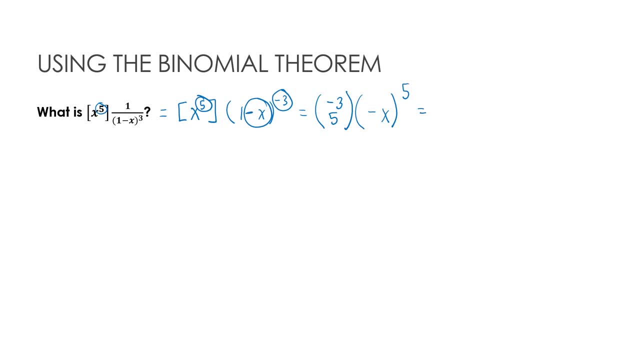 And this is going to be a negative x to the 5th. What I know about negative 3, choose 5 is that it's actually 3 plus 5 minus 1. Choose 5.. And then negative 1 to the 5th. 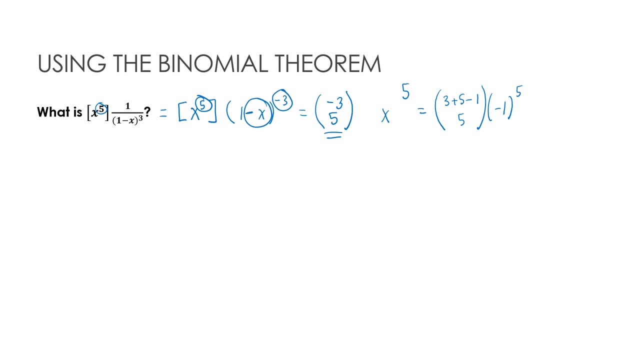 And what I know about. let's make this a different color. What I know about negative x to the 5th is that I really can write it as negative 1 to the 5th, x to the 5th. Now why does that matter? 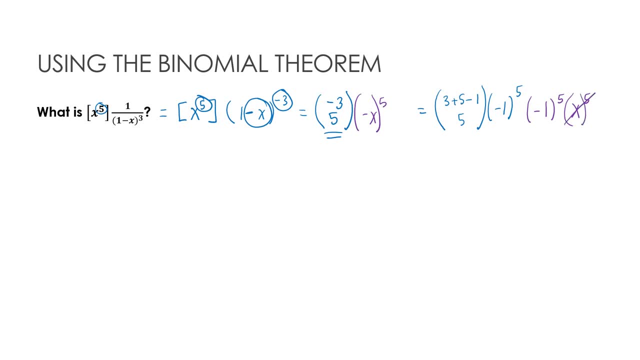 Because x to the 5th. do I care about it? No, It's not going to change my coefficient. It's just telling me that x to the 5th is going to be the variable value, And I'm only looking for the coefficient, which is all of this. 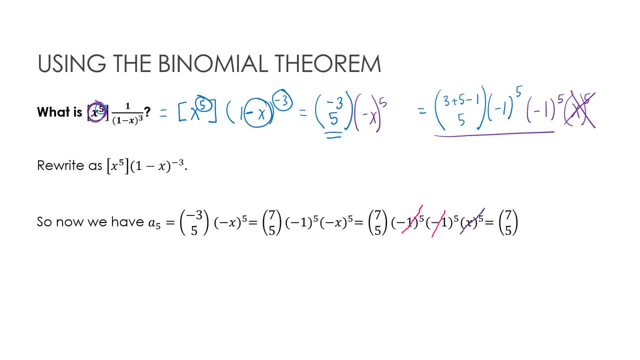 So, if you'll notice, negative 1 to the 5th is going to give me negative 1.. This is going to give me negative 1.. And negative 1 times negative 1 is positive 1.. So, if you'll notice, I've canceled out my negatives. 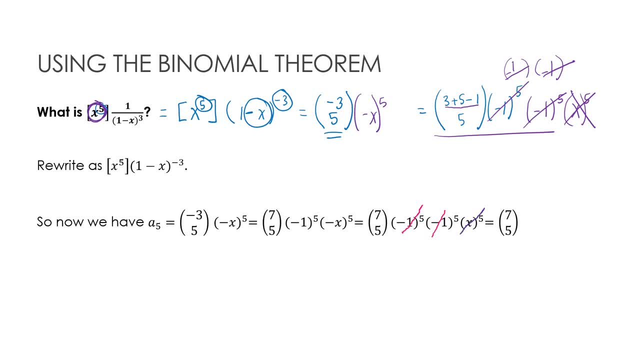 So really I just have 3 plus 5 minus 1, which is 7.. Choose 5.. That is my final answer. So again, we're putting all of this together to find 7, choose 5.. 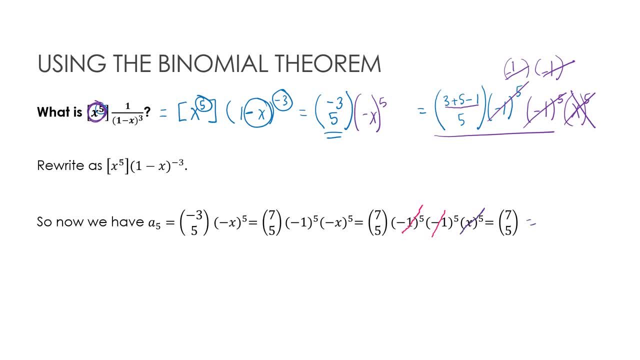 Now, if I were asked to, of course, I could find 7 factorial over 5 factorial, 2 factorial, which would be 42 over 2, which would be 21.. But typically 7, choose 5.. 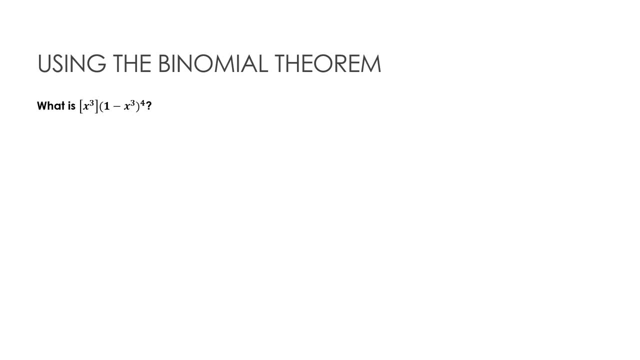 It's all I'll be looking for. Let's take a look at another one together. This one should be simpler than our last one. Notice here: this is n, This is k, So what I'm really looking for is 4. choose 3.. 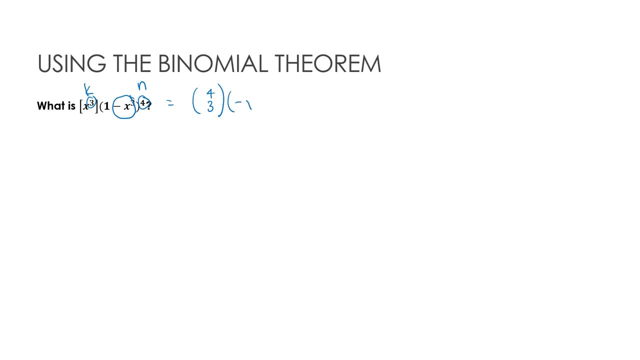 And because I've got a negative x to the 3rd or a negative x to the k power. this is really what I'm looking for And, just like before, I really don't care about the x to the 3rd. 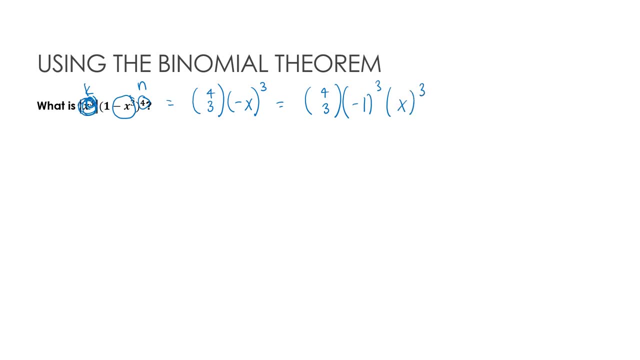 because that's just telling me that it's going to be the coefficient for x to the 3rd, So I don't even really need to write that x to the 3rd. So what this tells me is my solution is going to be negative: 1 to the 3rd, which is a negative. 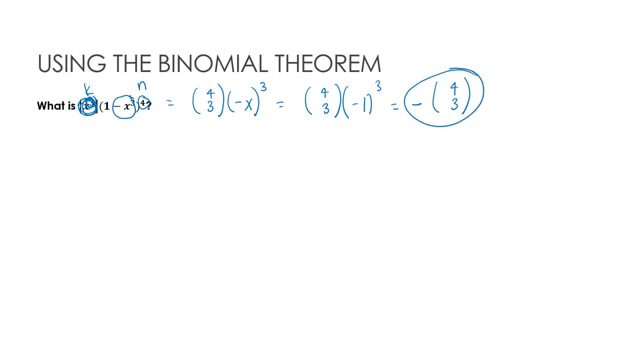 And then 4 choose 3.. That's my final solution. Now I've written some other things that will help us to look at just how we might write this Generally. So again I want to go back to where. did we start with this in section 9-1?? 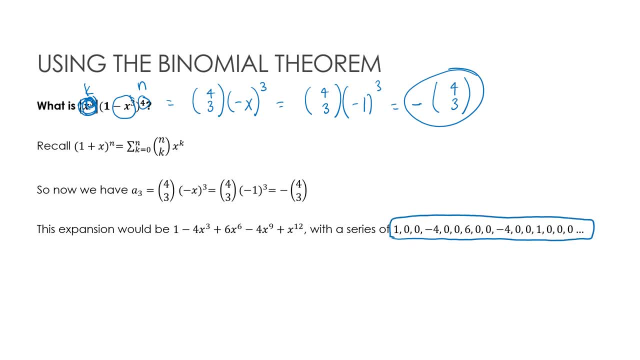 In section 9-1,. I gave you a list like this and said, hey, come up with a generating function. And we would have to come up with something like this. So I just want to kind of tie it back to where we started. 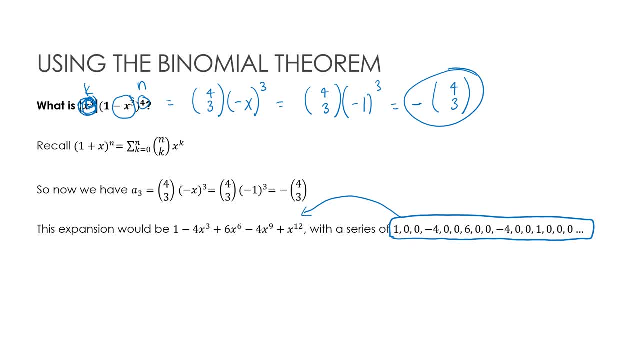 So you don't think I've completely gone off the rails here. This would be our expansion, going all the way through 12, because we've got 4 times 3,, which is 12.. And Again, we might even write this as a piecewise function. 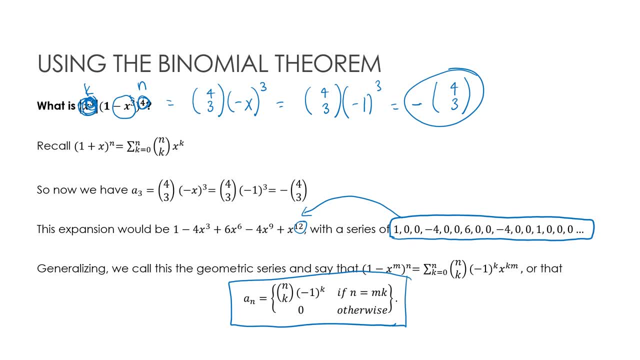 But really that part is not as important to me as you understanding right now just how to find the negative. 4, choose 3.. 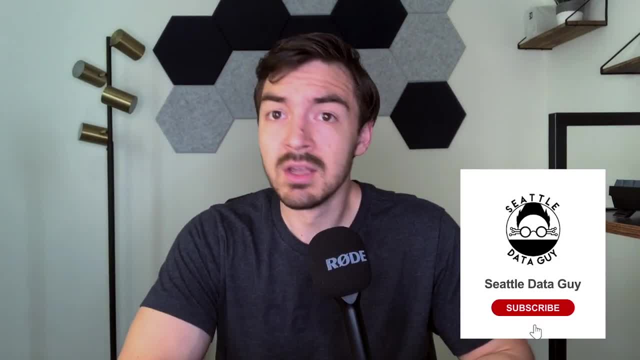 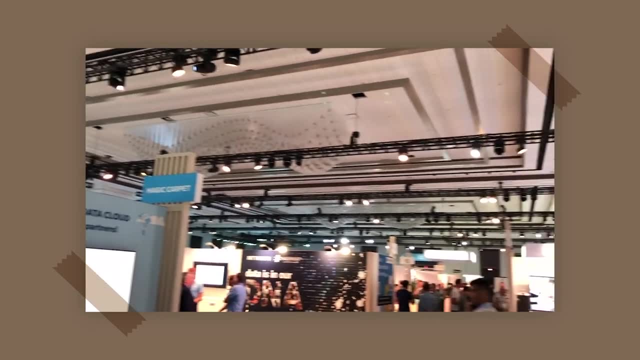 What is going on, guys? and welcome back to another video with me, Ben Roggenstein, aka the Seattle Data Guy. Well, as I just got back from the Snowflake Summit, I feel like it's only appropriate that I do a video about Databricks. 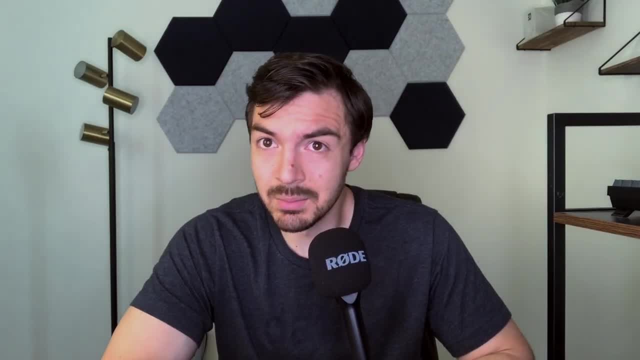 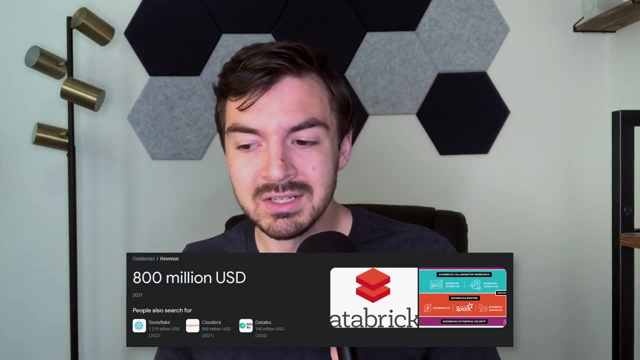 So the focus of this video is to answer the question: what is Databricks and why do people use it? When you look at the fact that Databricks is recording $800 million of revenue in 2021, it's got to make you stop and wonder. where in the world are they going to grow to? next? 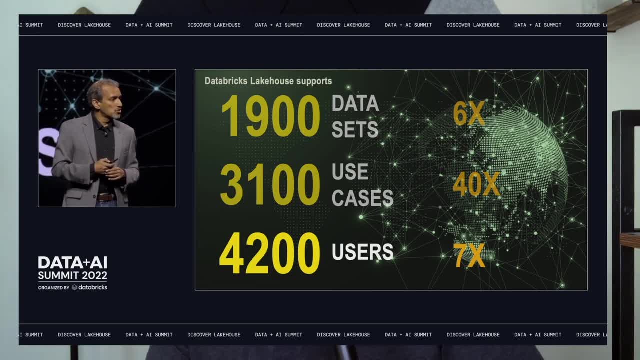 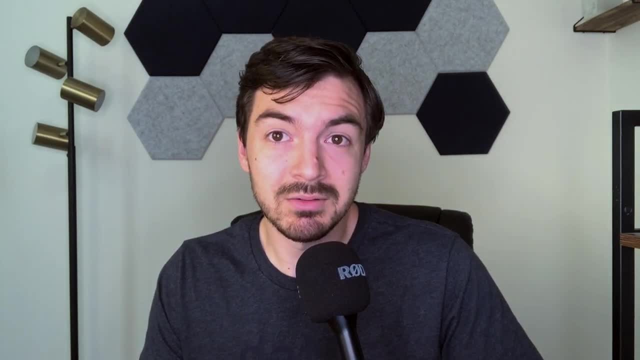 And since there have been a few times that Databricks has essentially passed the value of Snowflake based on their VC funding and valuation, it makes you wonder which tool is going to win out in this battle of what people are calling data lakehouses. 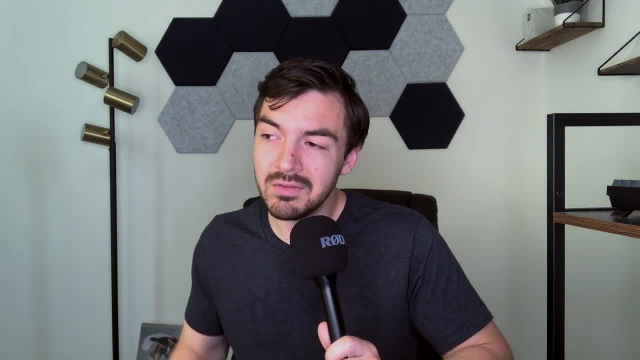 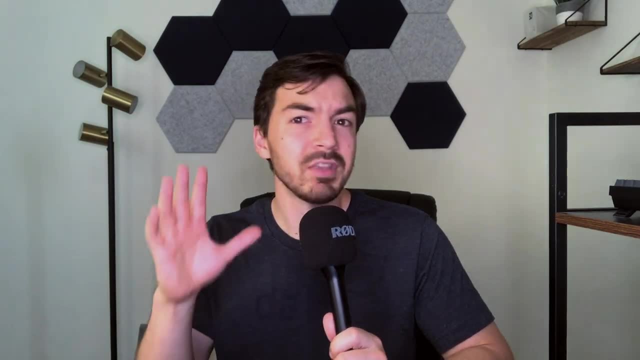 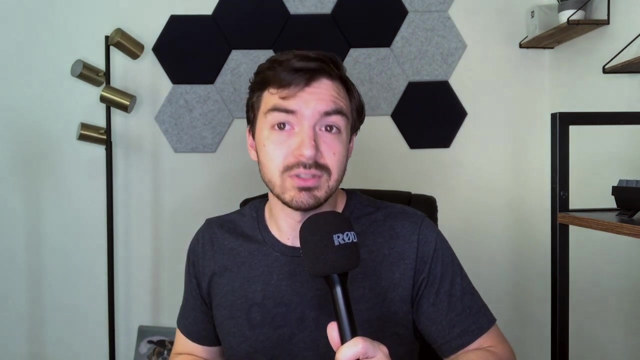 Now, arguably, that whole concept, I think, was brought out a little bit more from Databricks, but both solutions are trying to sell themselves as data platforms and not just a data lake or not just a data warehouse. So, on the cloud, they want you to know that they are so much more.